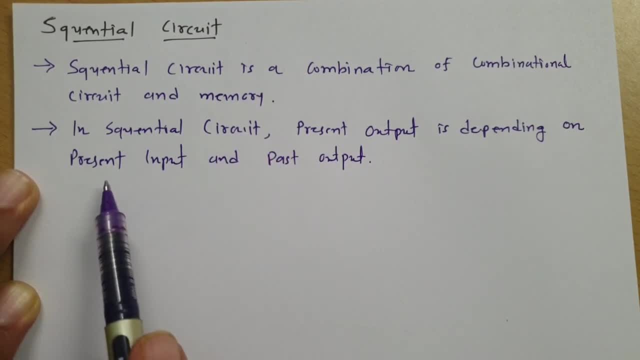 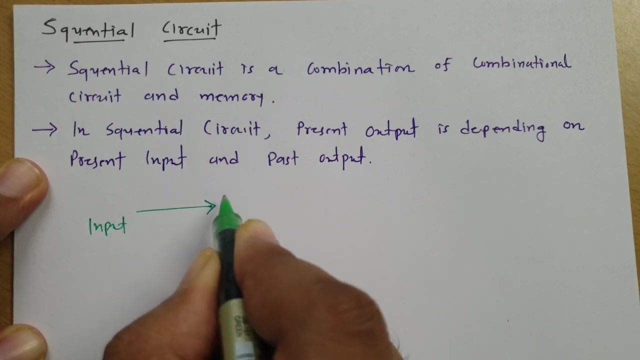 sequential circuit. present output is depending on present input and past output, And let us try to understand this by its basic block diagram. So it will gives you idea like how sequential circuit is functioning. So see, if I say I have input over here, So it is. 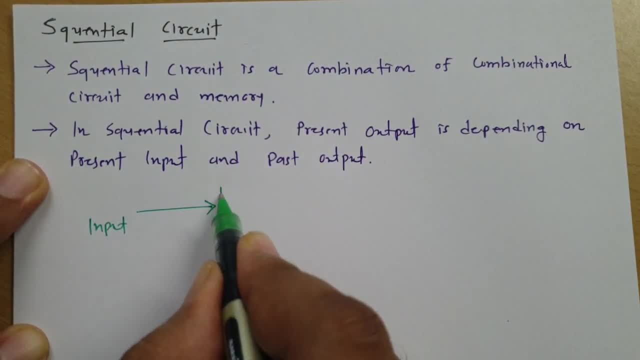 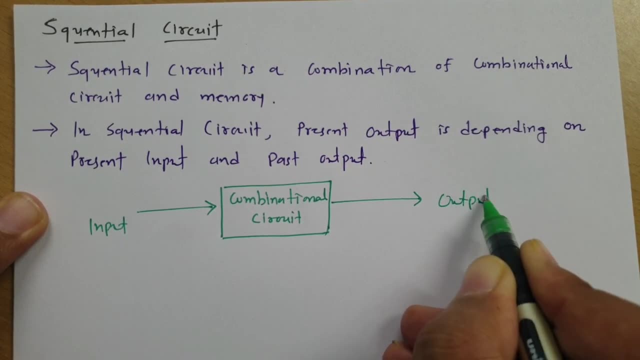 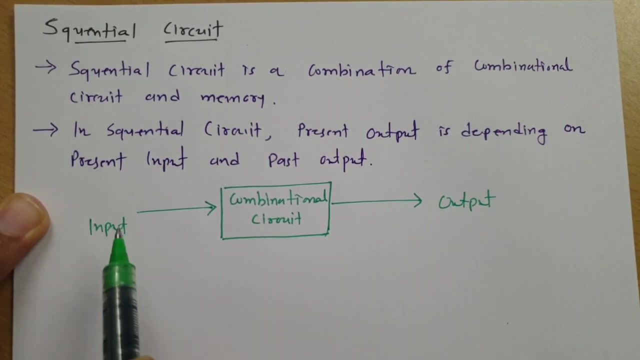 what combination of combinational circuit and memory. So here there will be combinational circuit. Here, if I say we have output, So this is where we are getting output. So as per combinational circuit, output is depending on present input. But here extra element, that 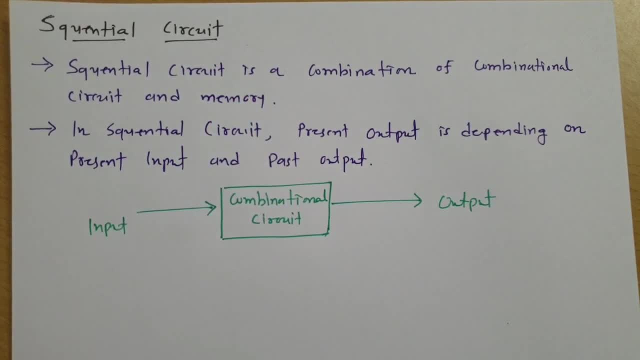 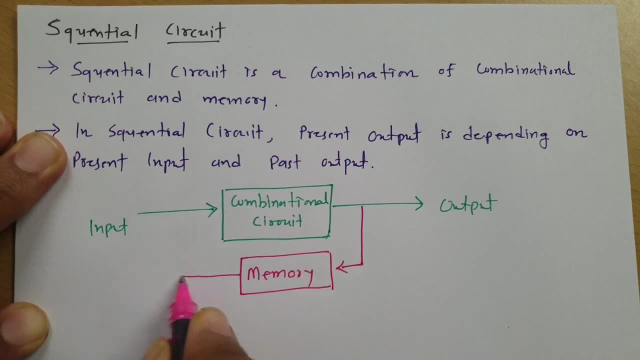 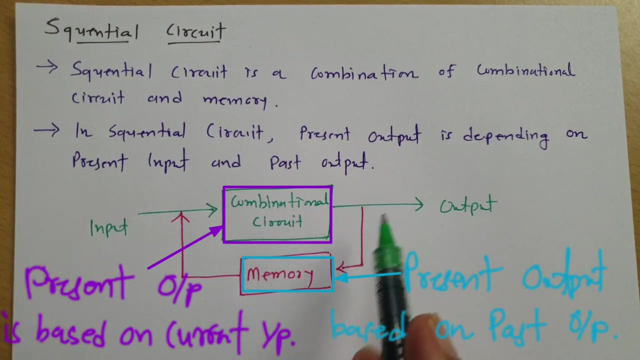 is memory which is there with us. So here we have memory in feedback. So see here output that is connected with memory. So because of this memory, Now your present output that is depending on current input as well as past output. You see, in feedback we are taking memory. So your present output that is depending on past output. 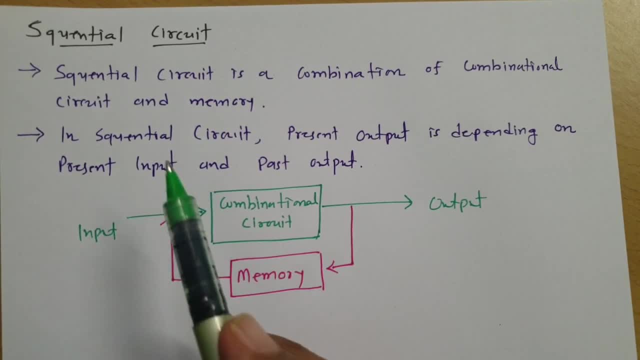 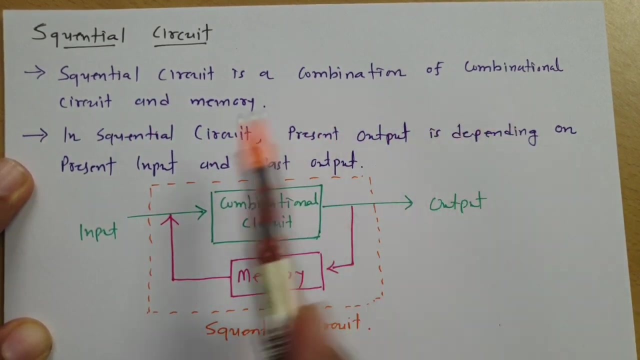 as well as present input. So this is how sequential circuit basic block diagram is there. So one can say: this is what resultant block diagram of sequential circuit. So these are the basics that one should know. Sequential circuit is a combination of combinational circuit and memory and its present output. 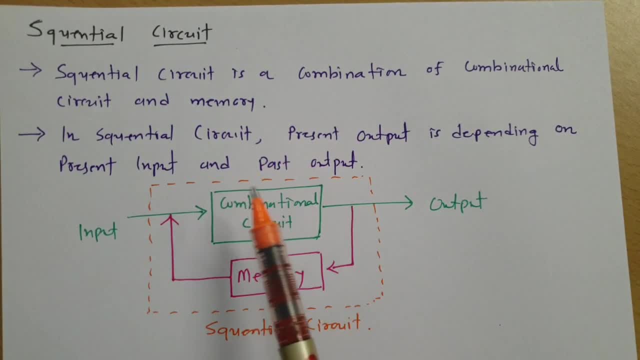 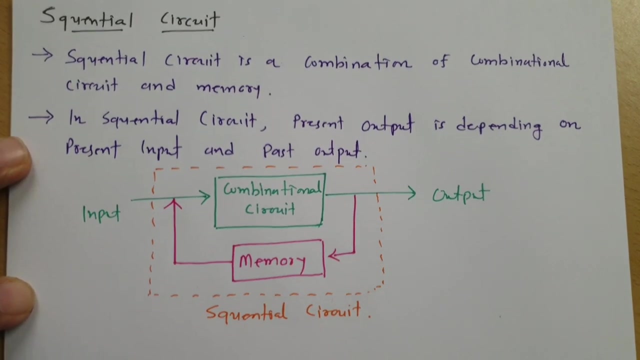 is depending on present input and past output. So past output, dependency on present input, that is there because of this memory elements that one should know- And combinational circuit results, output as per current input. Let me give you some practical examples of sequential circuit So that will gives you idea, like what are the examples? which is there with 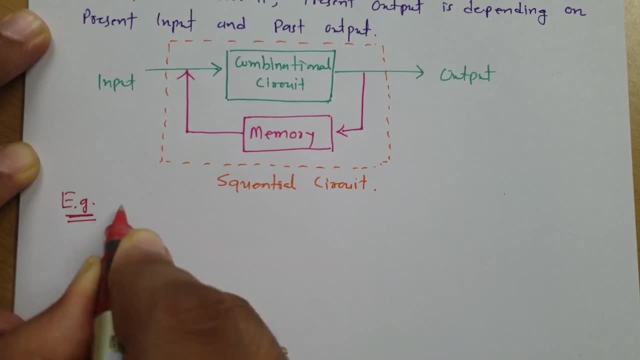 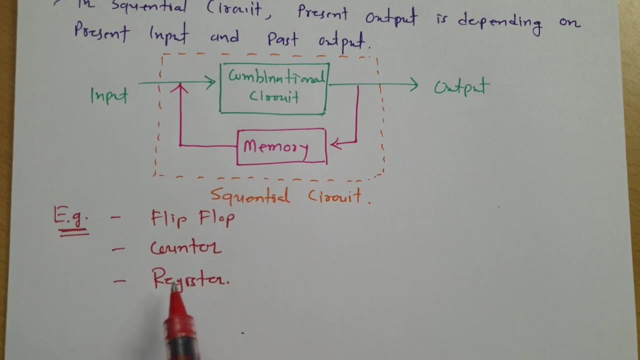 sequential circuits. So examples of sequential circuits are like flip-flop, like counter, like resistor. So see, these are the basic examples which is there with sequential circuit and all these examples that I will be explaining in detail. So you will get to know like how those flip-flop 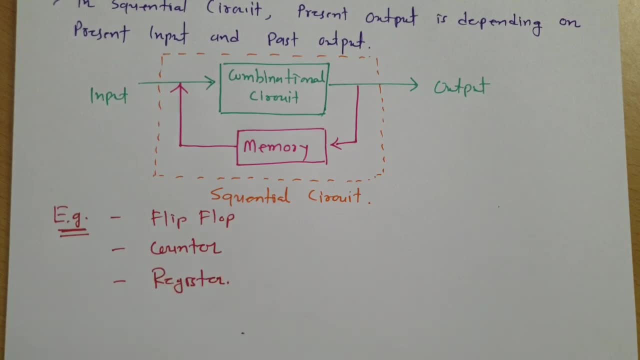 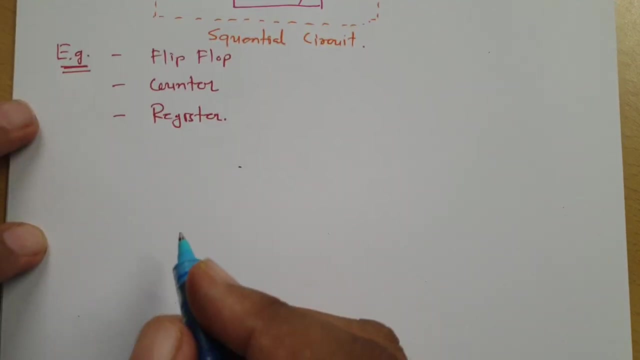 counter and resistors are functioning in sequential circuit. Now I will give you classification of sequential circuit. So one can classify sequential circuit in two parts. One is synchroneural potential circuit and second is Brenne, A synchronous sequential circuit. So let me mention it So sequential circuit that can be classified. 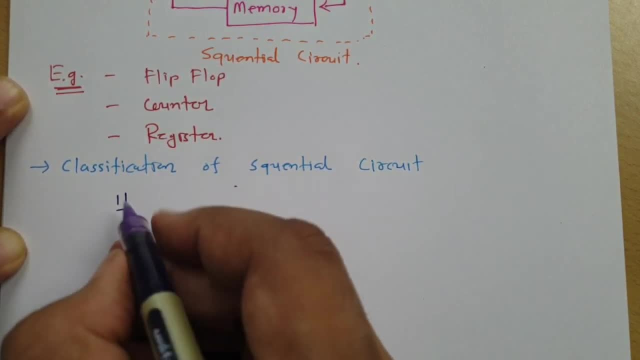 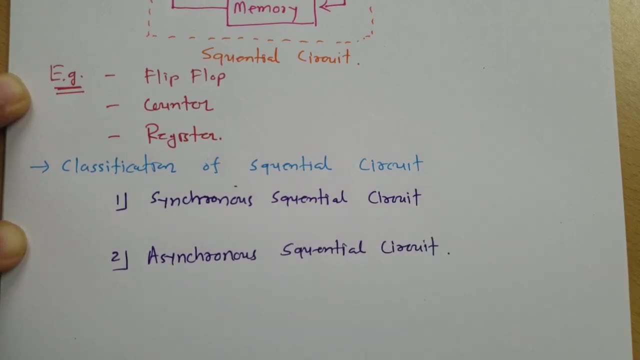 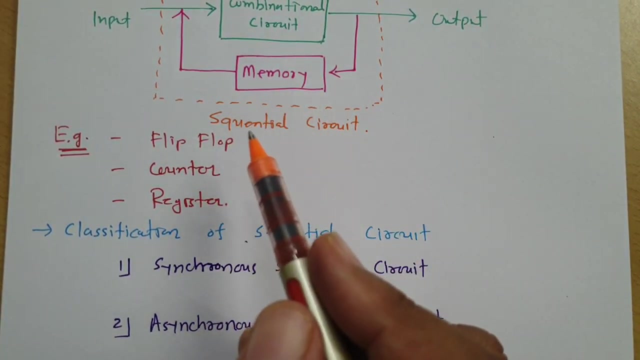 in two parts. One is synchronous sequential circuit And second is a synchroneural sequential circuit. Now let us try to understand what is the meaning of synchronon sequential circuit. See, in sequential circuit you will be using memory element. So in memory element usually we use flip-flop and those flip-flops are required to have. 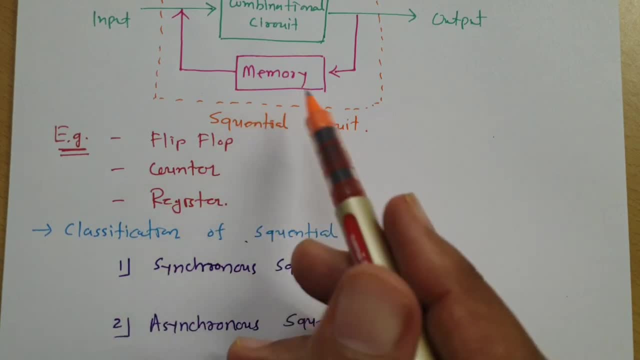 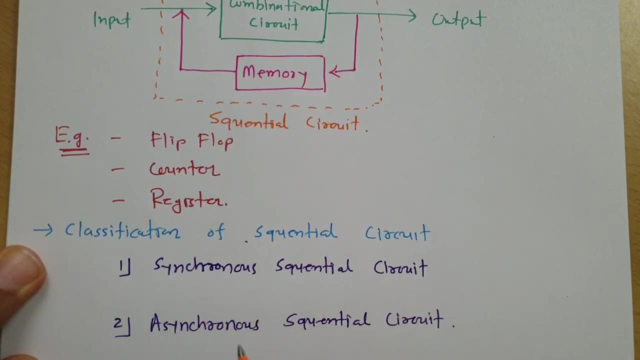 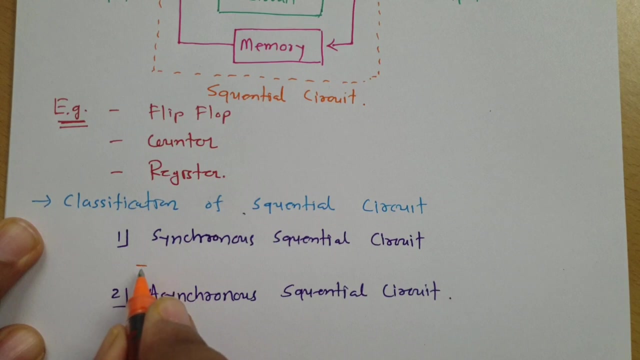 input as a clock frequency, So clock signal, that is what required to operate with memory element. and in synchronon sequential circuit you will be finding all memory element that will be given with same clock. So in synchronon sequential circuit all memory element that will be given with same clock. 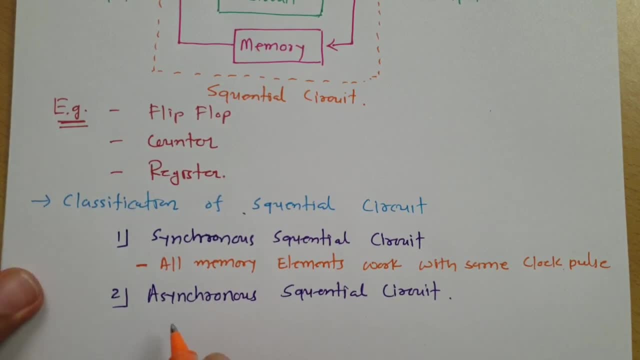 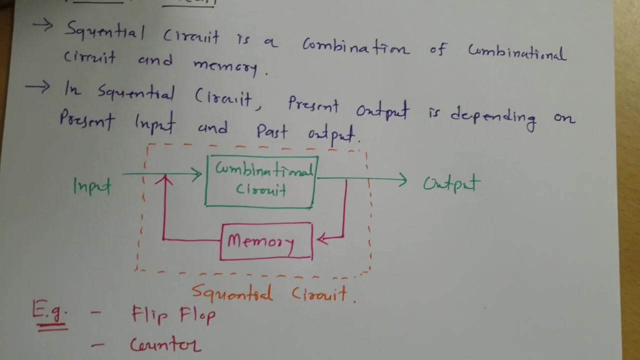 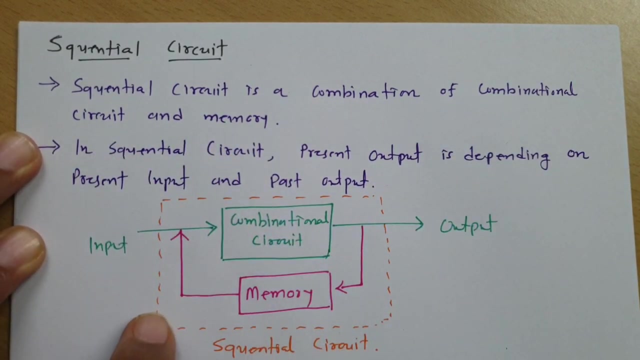 and in asynchronous sequential circuit you will be finding memory elements are functioning with different clock pulse. So this is how we can classify sequential circuit. So let me give you quick review again So it will gives you bit better idea. See sequential circuit. that is a combination of combinational circuit and memory. 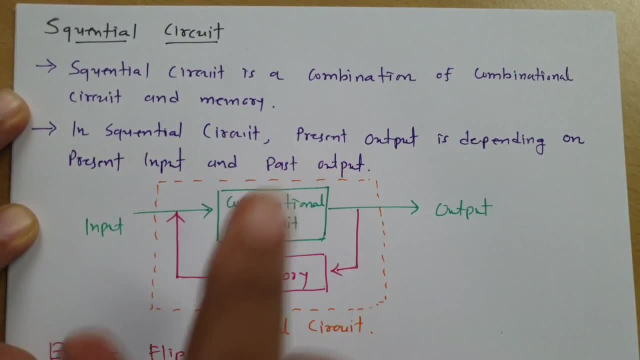 In sequential circuit present output is depending on present input and past output. So if you observe combinational circuit, then combinational circuit output is only depending on present input. but in sequential circuit we have additional elements. that is memory. So because of memory, our resultant current output. 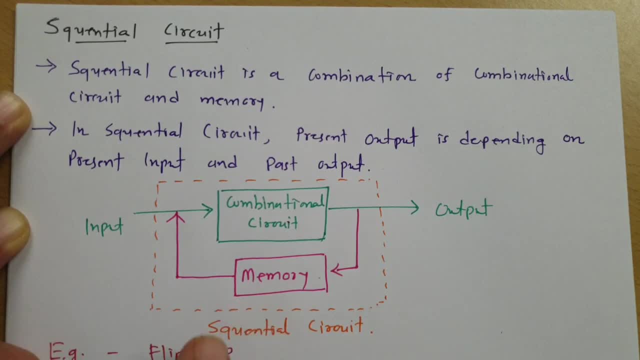 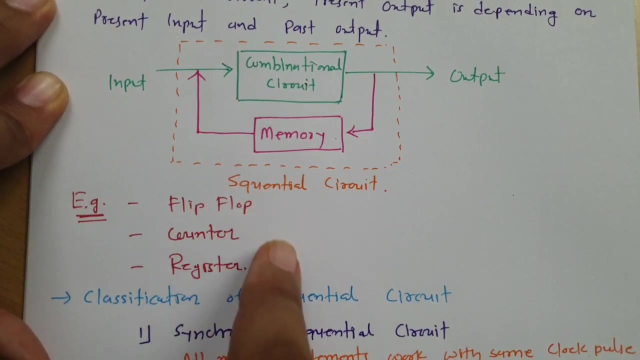 That is depending on past output also. So we can say all together in sequential circuit, present output depends on present input and past output. Few examples that I have listed here: we will see it in detail in future videos: flip-flop counter and resistors.